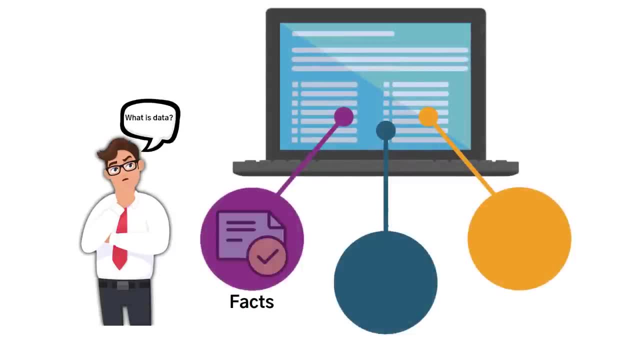 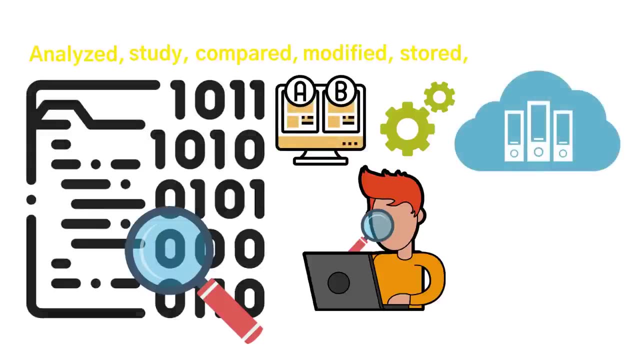 exactly is data? Data is every type of information, from facts, statistics, numerical sequences and patterns- which is analyzed, studied, compared, modified, stored and, overall, used as a component in the overall environment of the world. So what exactly is data? Data is every type of information. 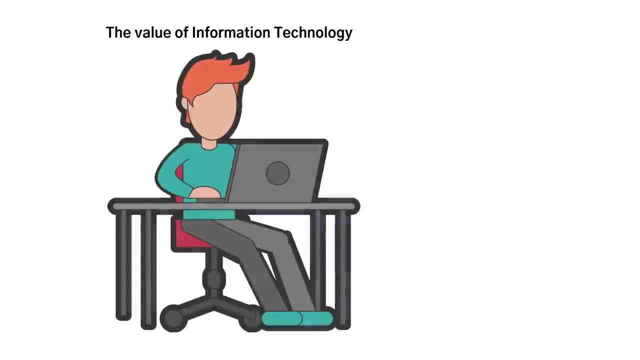 and patterns, which is analyzed, studied, compared, modified, stored and, overall, used as a component in the overall environment of the world And the overall information that the technology user needs. The value of information technology is that, although people are capable of handling data using our brains and even the old paper and pen processes, 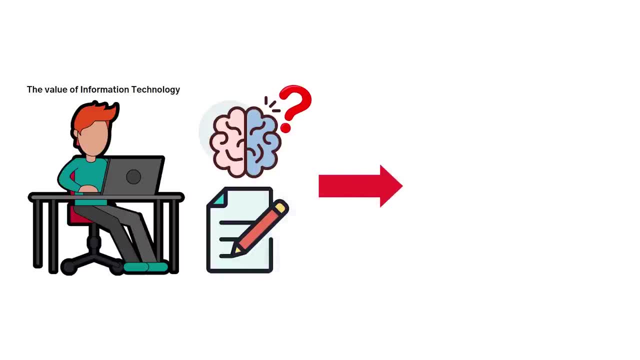 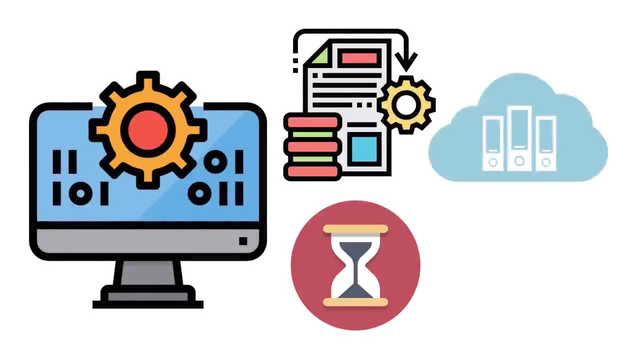 these processes are not as reliable, efficient and effective as relying on information technology. A computer can process millions of pieces of data at a given time. Its storage or memory can hold and secure information without forgetting a single piece of data. So where is information technology? 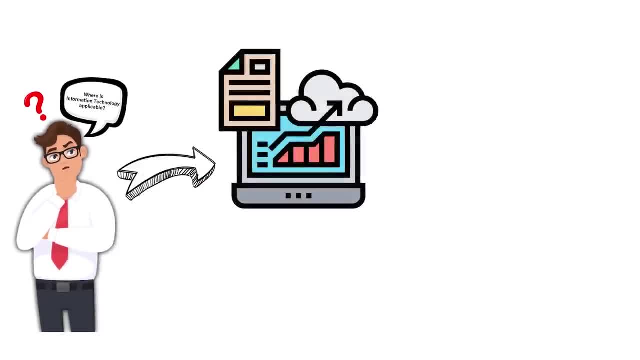 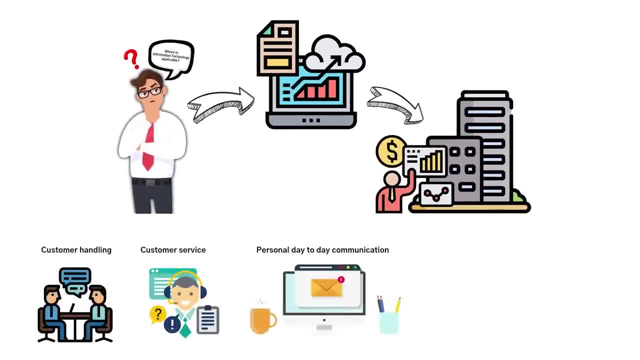 applicable From the general information above, information technology plays a significant role in business. Some examples of this would be customer handling, all the way from handling customer service, personal day-to-day communication, storing financial records and all other human activities that deal with handling electronic data. Information technology is essential to the 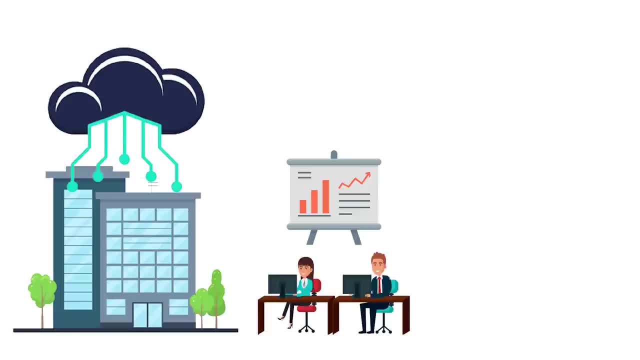 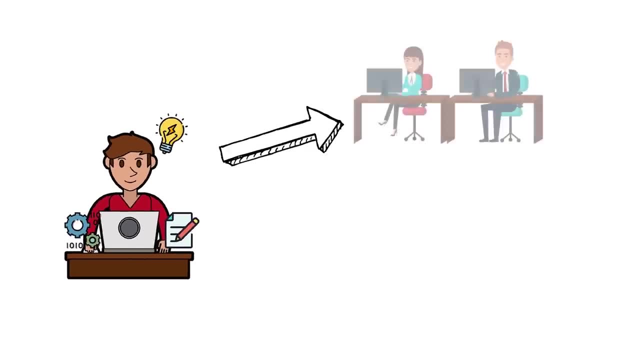 day-to-day operations of a business, and, even more important, when it comes to scaling your business to make more money, And this is why learning the skills of information technology is incredibly valuable, whether you want to get a job or start your own business. Next, let's talk about hardware versus. 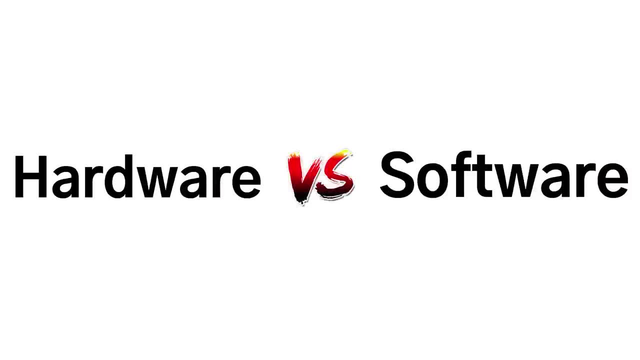 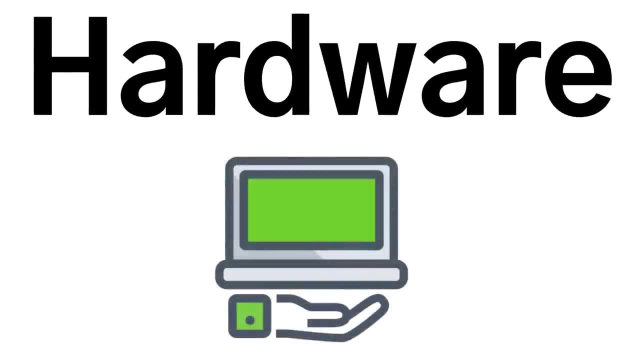 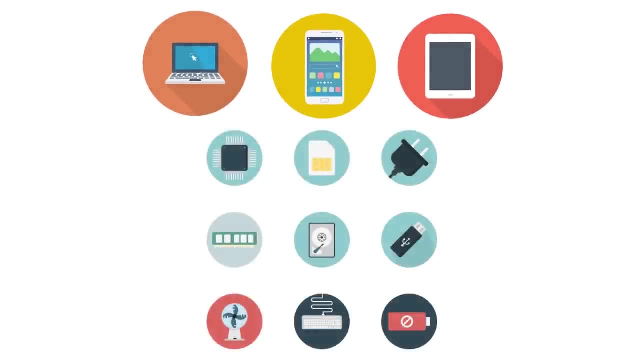 software. Before we can discuss examples of information technology, it's important that we talk about hardware and software. Hardware is tangible technology that you can actually touch when it comes to dealing with information technology from personal computers, laptops, mobile phones, tablets and everything else that is physical and is used for the purposes of IT. 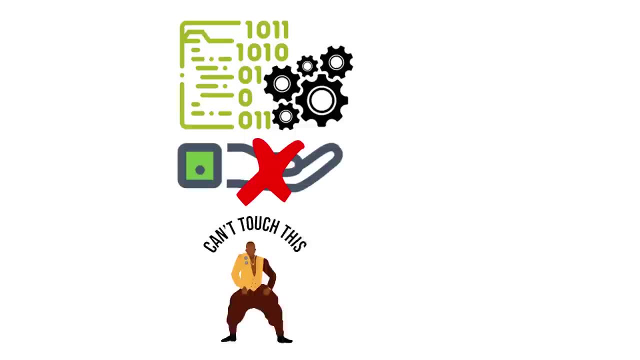 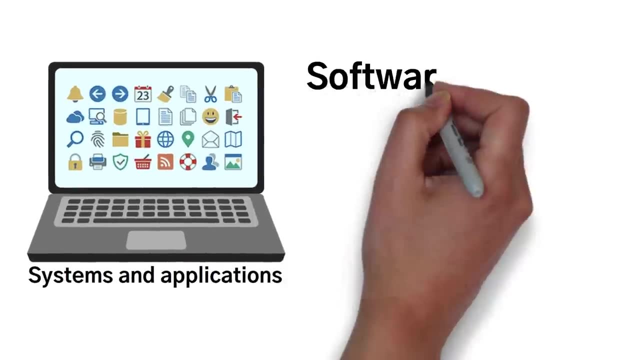 Software, on the other hand, is intangible, aka you can't touch it. So this would be things such as websites, computer programs or systems and applications, And it's going to be broadly separated into two different groups, which is software systems and software technology. 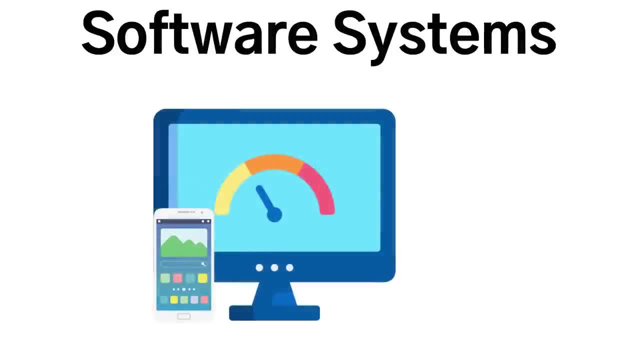 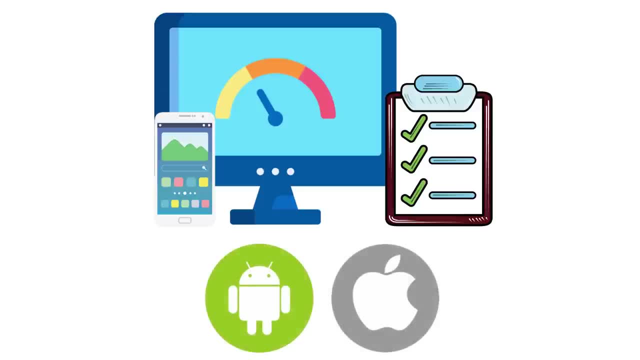 Software systems are basic programs that are tasked to perform computer functions at its most basic level. An example of this would be an operating system for a phone such as iOS or Android. Applications, on the other hand, also have a lot of examples, such as databases.